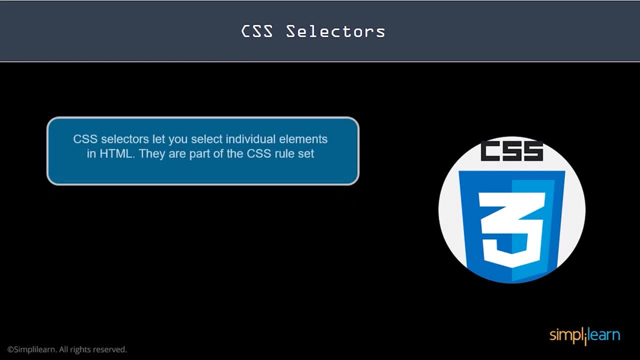 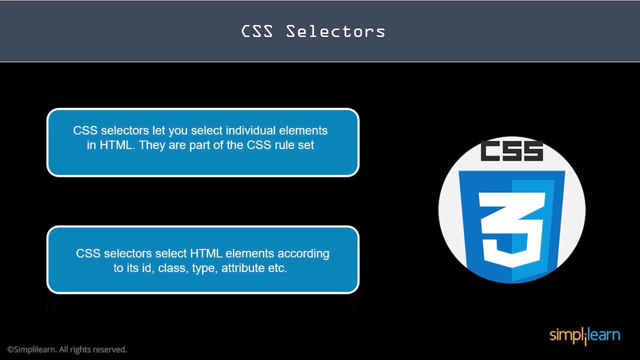 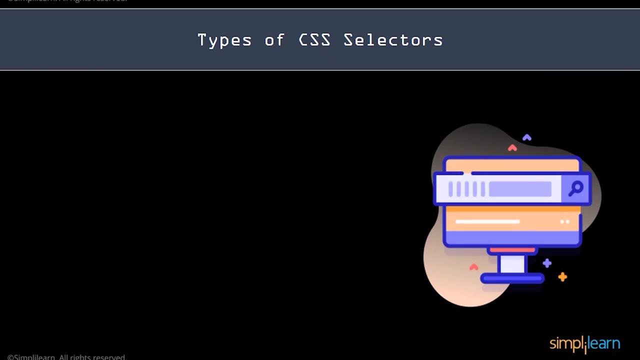 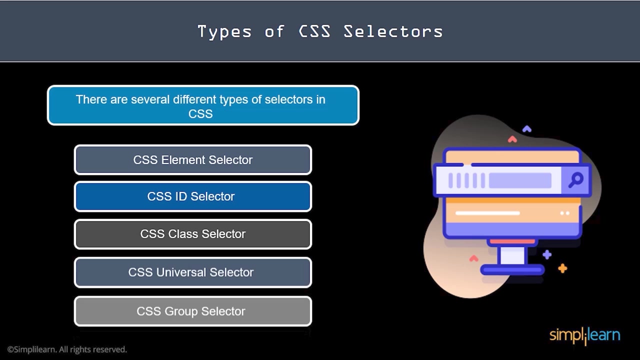 So what are CSS selectors? CSS selectors allow you to select and style HTML elements. Selectors are used to find elements based on their ID, classes, types, attributes, value of attributes and much more. Let's discuss the most common selectors. There are several different types of CSS selectors. The most common of them are CSS element selectors, CSS ID selector, CSS class selector, CSS universal selector and CSS group selectors. 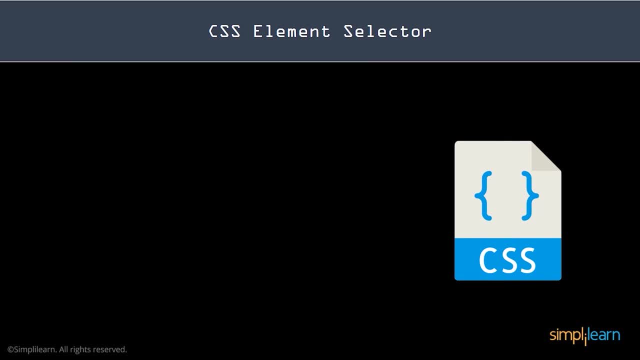 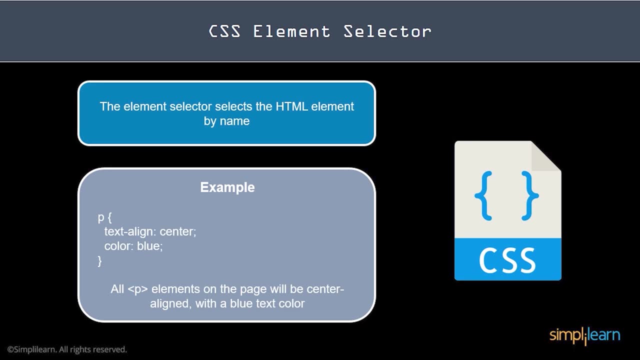 So what is a CSS element selector? The element selector selects elements based on the element name. This is a CSS selector. It means it will select all the P elements on the page. It will style all the P elements to the center, aligned, having blue color. 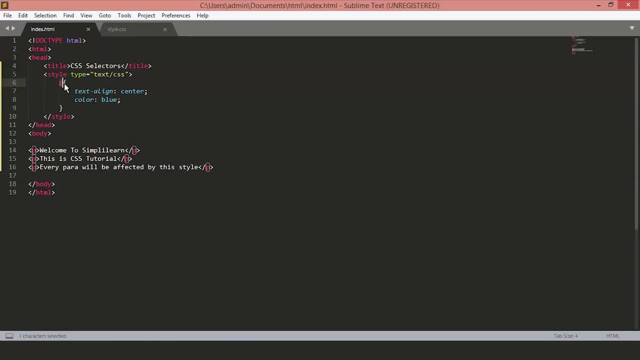 This is a CSS selector. It is set to P. This means it will select all the P elements on the page. It will style all the P elements to the center, aligned, having blue color. Let's look at what it looks on a page. 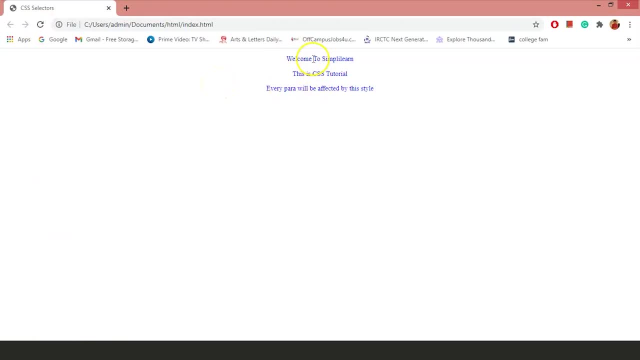 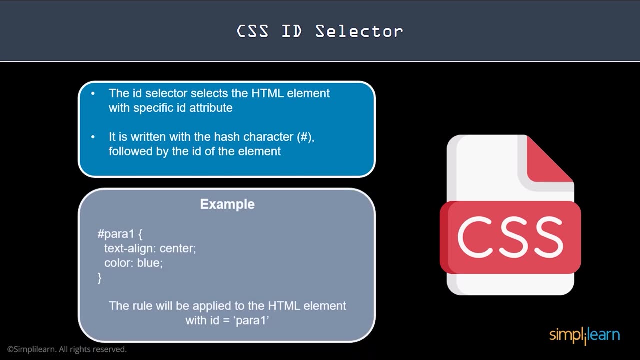 So, as you can see, all the elements are centrally aligned with a text color: blue CSS ID selector. The ID selector uses the ID attribute of an HTML element to find a specific element. An ID should be unique within the page, So you should use the ID selector to find a single unique element. 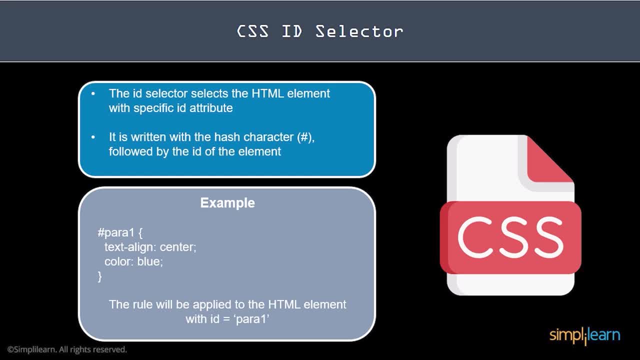 To find an element within a specific ID, use a hash character followed by the ID of the element. So here we have used the hash paraben, So all the rules will be applied to the HTML element with ID equal to paraben. 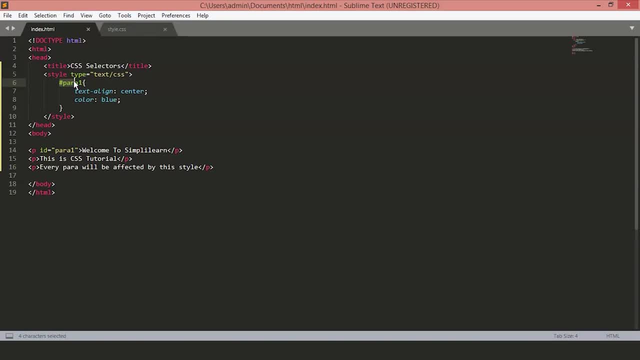 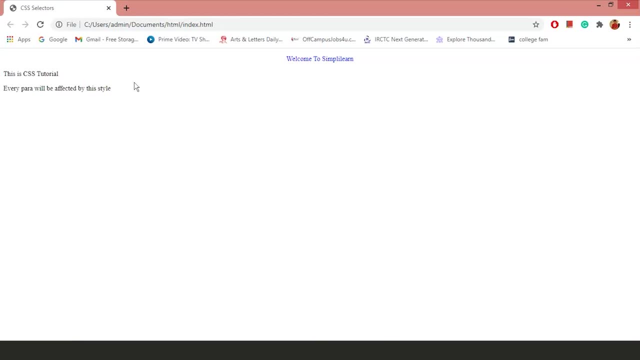 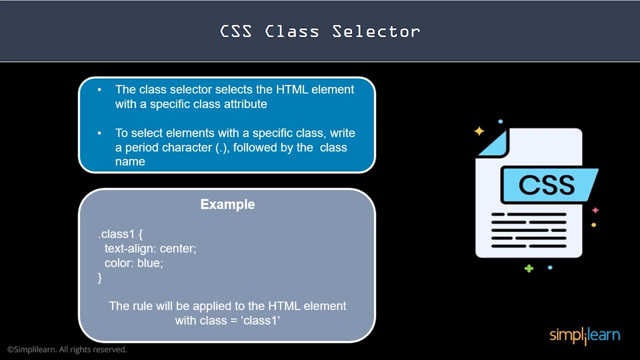 So this is an ID selector. It will be applied to all the HTML elements with ID equal to paraben. As you can see, it is applied to the element having the ID paraben, and all the other elements are defaultly styled. CSS class selector. The class selector finds the element with a specific class set by the HTML class attribute. 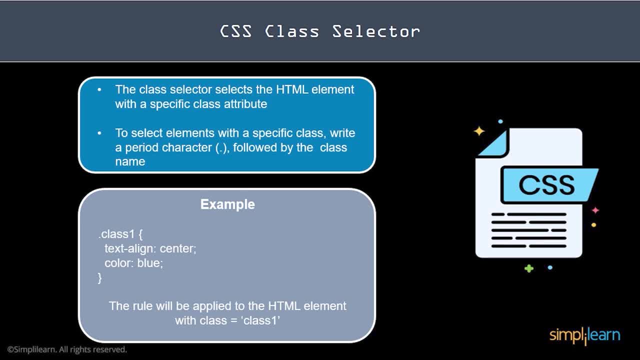 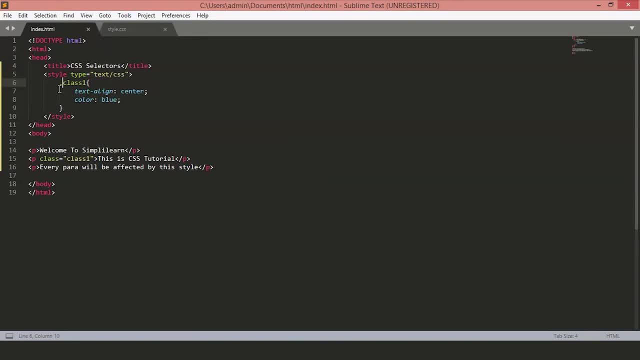 To select an HTML with a specific class, use a period character followed by the name of the class, So this style will be applied to all the elements having the class name class1.. This is a class selector. It is denoted by a period symbol.